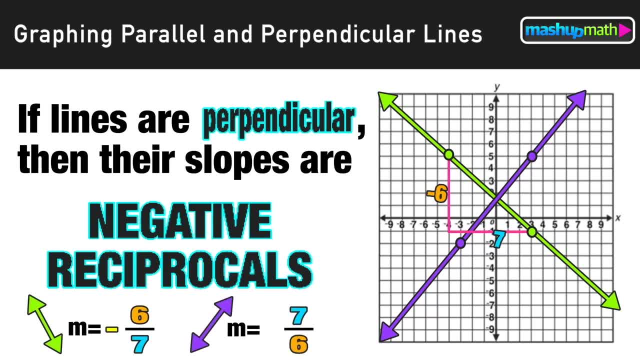 And again, what that means is flip and switch. We take the slope of the other line, we flip it and we switch the sign. So in this case now it becomes positive 7 over 6.. Now you're probably asking: why did we do that? Let's take a look at the slope of the purple line. 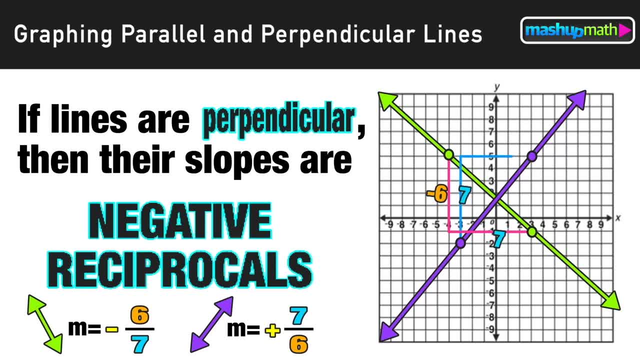 now, If we go from point to point, we're rising up 7 units and then we're moving to the right 6. And this negative reciprocal relationship between the slope of two lines will end up in those two lines being perpendicular to each other. 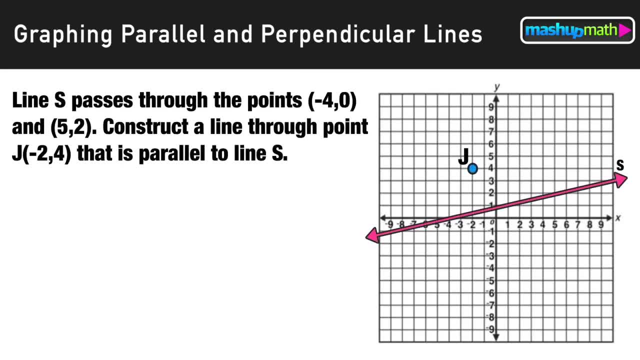 So now we'll look at a few examples where we have the opportunity to apply these concepts. So on this graph, we are provided with a line S that passes through the points and positive 5, positive 2.. We're also provided with a point J with coordinates. that is not. 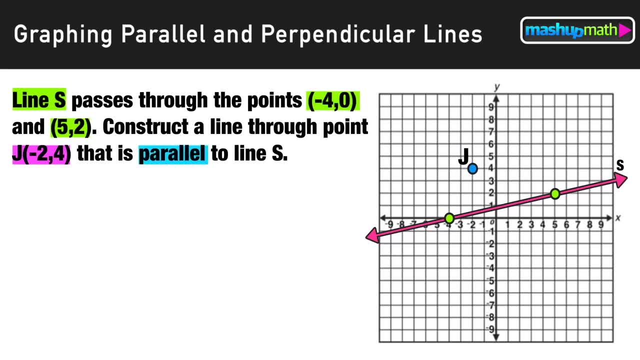 parallel to the line. Now our goal is to construct a line that goes through point J, that is, parallel to line S. Now the word parallel should tip us off to thinking same slope. So we can go ahead and find slope the easy way, just by calculating rise over run. We should notice. 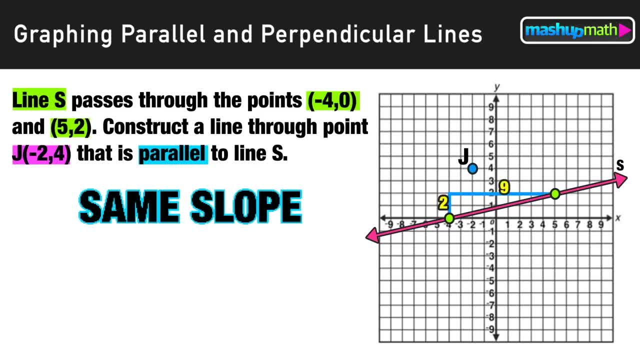 that, moving from point to point, we're moving up 2 units and to the right, 9.. So the slope of line S is 2 over 9.. Now we know that our parallel line will have the same slope. So we're going to repeat that slope, starting from point J, by rising up 2 units and then 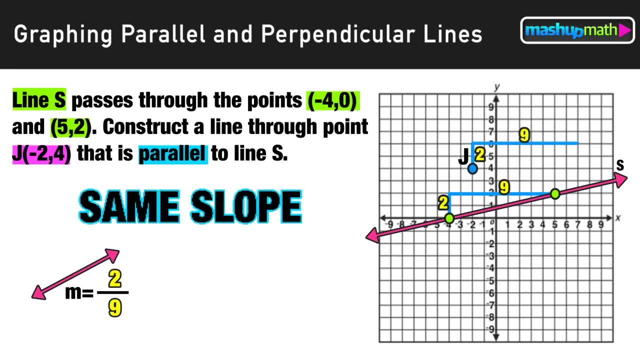 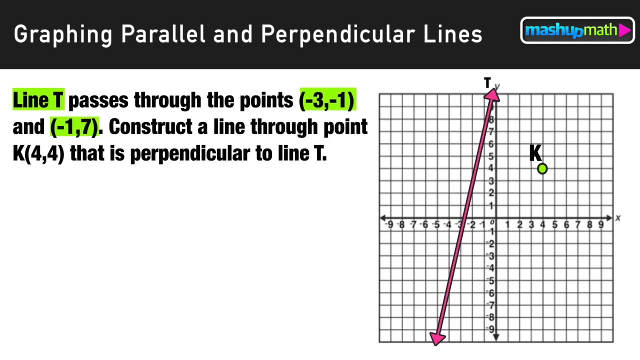 running to the right 9 units and then plotting a new point, And finally, all we need to do is construct a new line through those two points that is parallel to line S, with a slope of 2 over 9.. Okay, let's look at a different example now. Here we have a line T passing through two 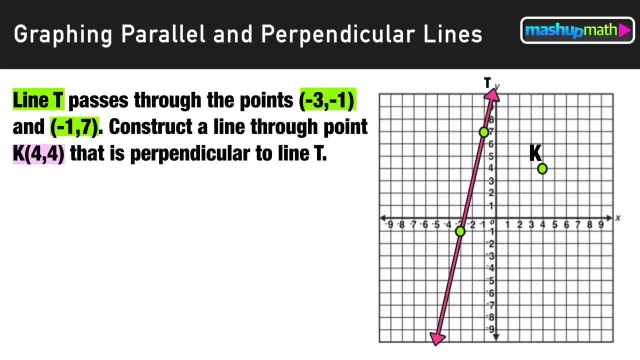 points. We have negative 3, negative 1, and negative 1, positive 7.. We have a point K that is not on the line And we want to construct a line that is perpendicular to line T that passes through that point K. So when we see perpendicular we need to think negative reciprocal slopes.